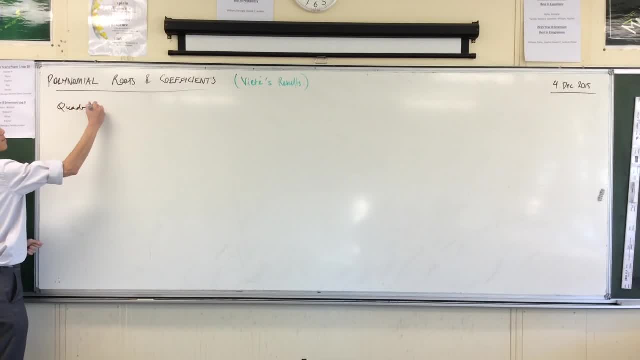 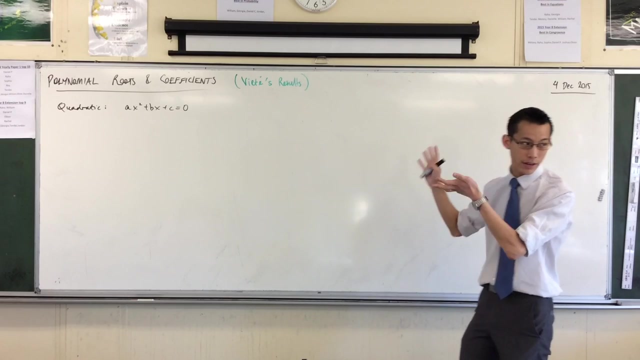 For a quadratic right. we can state any quadratic polynomial as like with general coefficients in general form, right. So if I have ax squared plus bx plus z equals zero. okay, Out of this I can make a statement if I say the roots are alpha and beta, because it's a quadratic so it should have two roots. 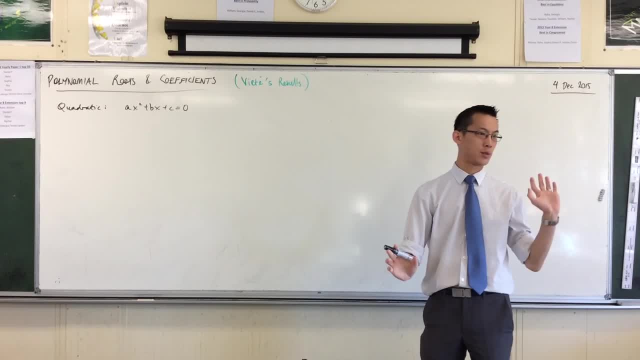 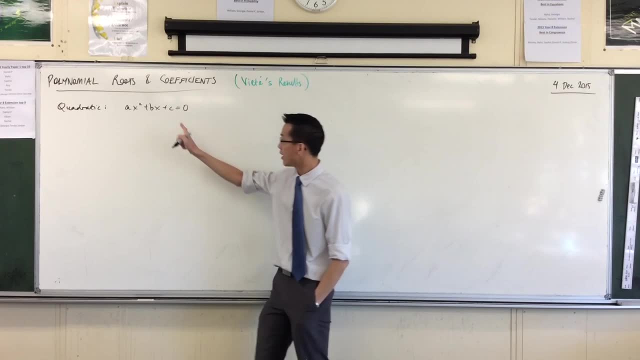 I can make a statement about what happens when I add those roots and what happens when I multiply those roots. right Now, if you recall how we got this relationship, what we said was: look if I've got a quadratic like this, and you don't need to rehearse this. 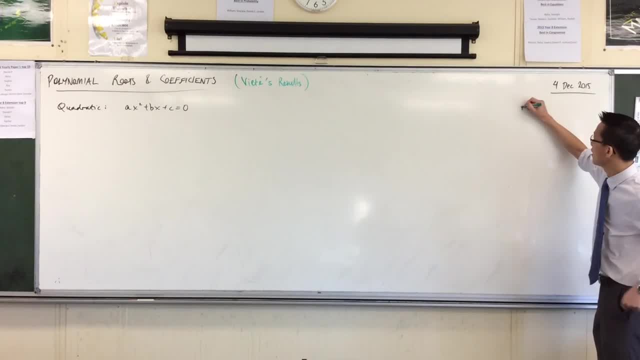 I'm just going to say this, right, I'm just going to do it quickly on the side and we're going to do it for a cubic and a quartic. If you have a go at something like this and you say, look this quadratic, it ought to have two roots, right. 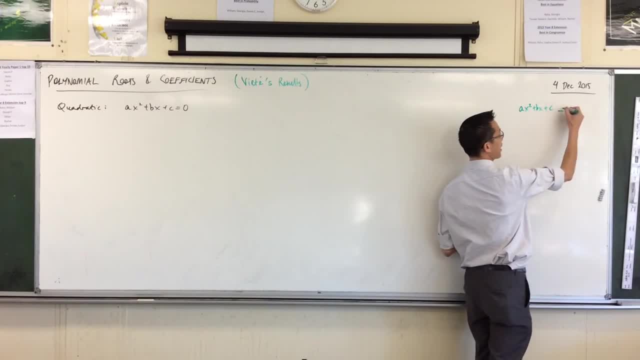 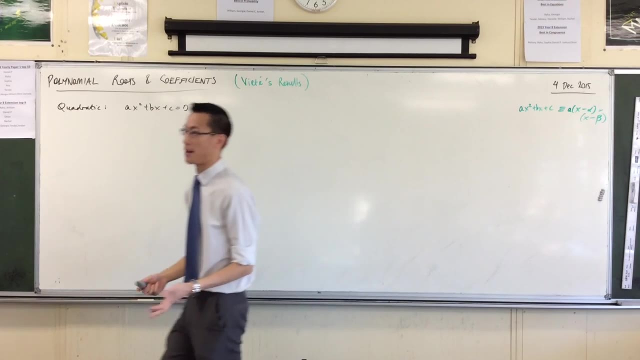 It ought to have two roots. I should be able to say that I could rewrite this, not say it's equal to something, but actually say it's identical to a quadratic. that looks like this: Oops, not enough space. Okay, It's got two roots, alpha and beta, and I can't just say x minus alpha, x minus beta. 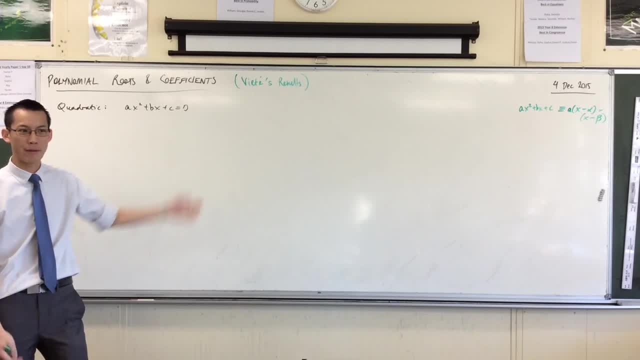 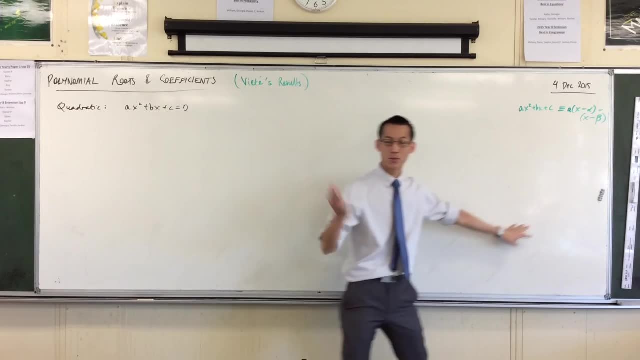 and say that's the factorization, Because I don't know whether it's monic or not. A could be 1 or 2, or negative 100 or anything. okay, So that's why it's at the front. okay, Now what I would do here, just like we did in so many places, right, 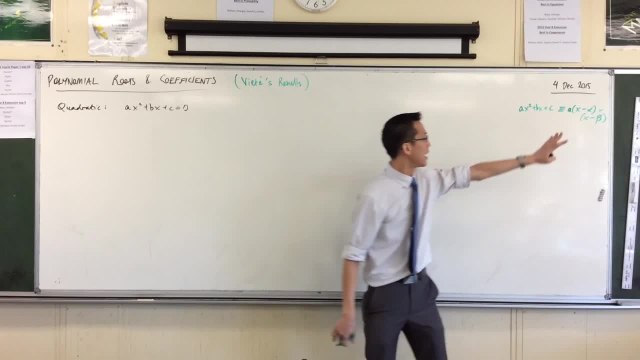 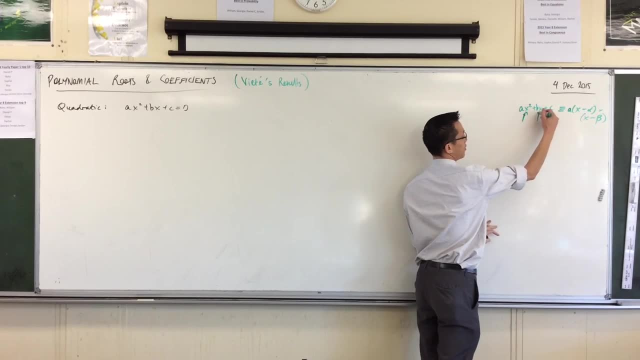 Because we're approaching the one object from two points of view. okay, I'd expand the right-hand side and then I'd have some x squared terms, some x's and a constant, just like I have here, And since these things are identical, I would equate them. 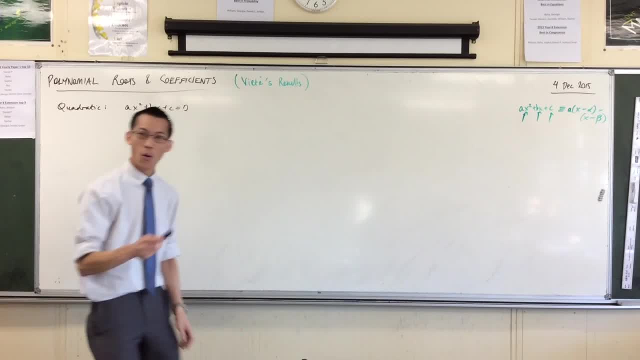 I'd compare coefficients and then I'd get a result out. Now let's just rehearse. What is that result? What is the sum of the roots of a quadratic Minus b and a, Minus b and a? very good, 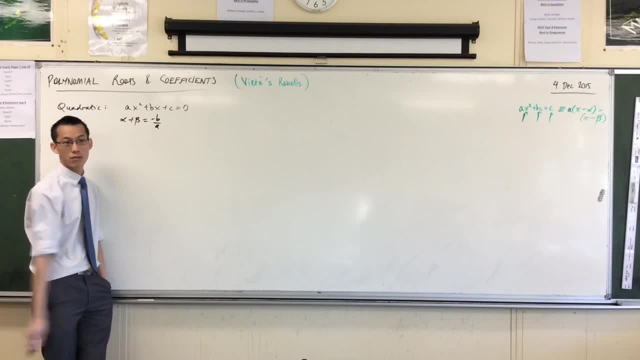 Cool, Right, There's the sum of roots and in the same way, once you rehearse that process, you get the product of the roots, alpha times, beta, which is C on a, Just c on a right. So a couple of things have happened. 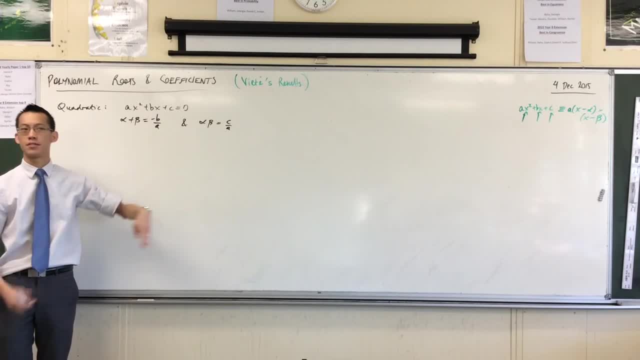 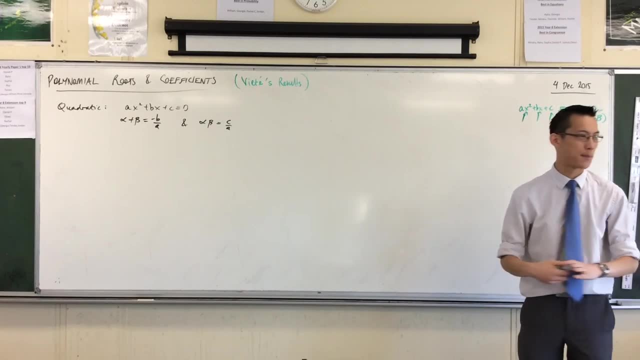 Number one. the coefficient has changed and also it's gone from negative to positive. No big deal, okay. Sum and product of roots. Now, as it turns out, sum and product are actually not a very real thing. It's a very appropriate name, as you will see, as we now generalize this result, okay. 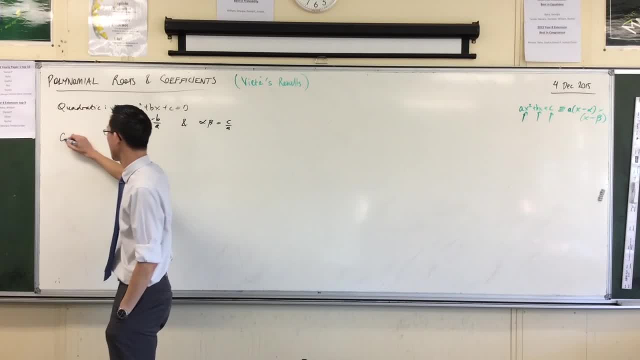 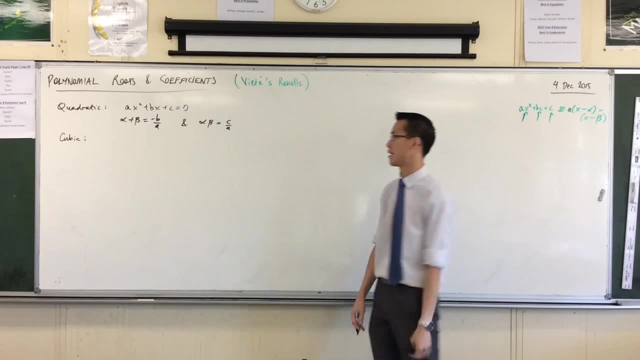 So now, rather than just a quadratic, we're going to have a look at a cubic, And this time we are going to fully rehearse this result rather than just say, hey, do you remember this? We're actually going to go through the lines, okay. 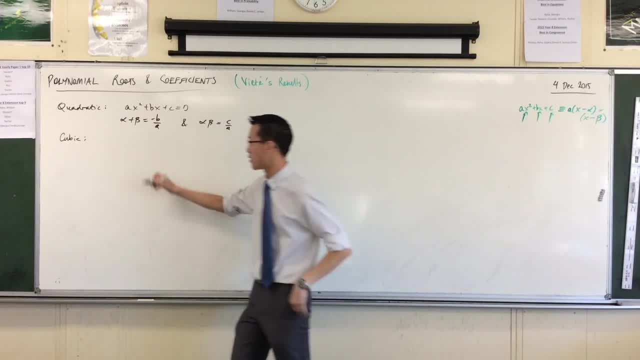 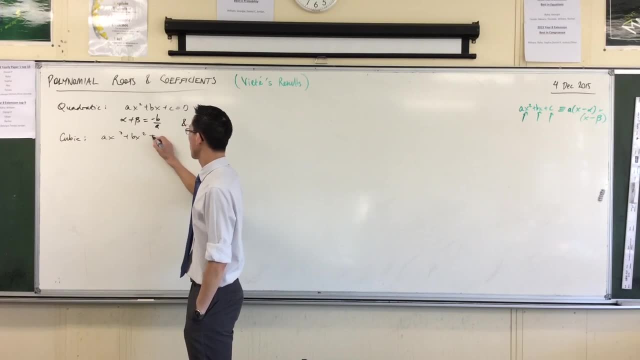 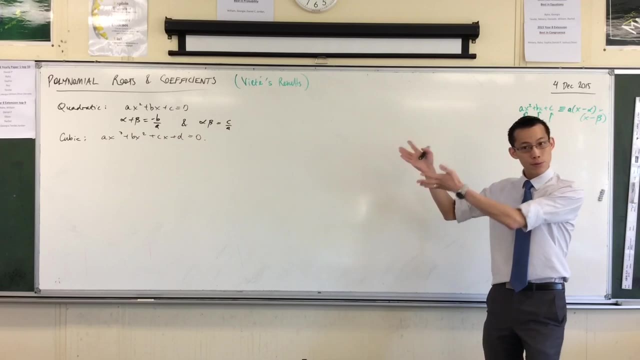 So I'm going to say we're going to start with a general cubic. right Again, I'm going to name the leading coefficient a. so I've got ax cubed plus bx squared, plus cx plus d. Now what I want to know is something about the roots of this cubic, and how many roots should it have? 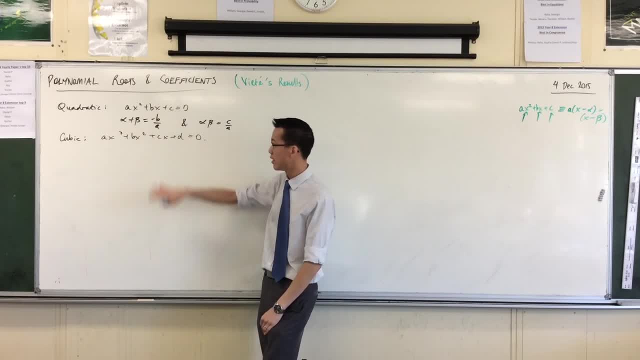 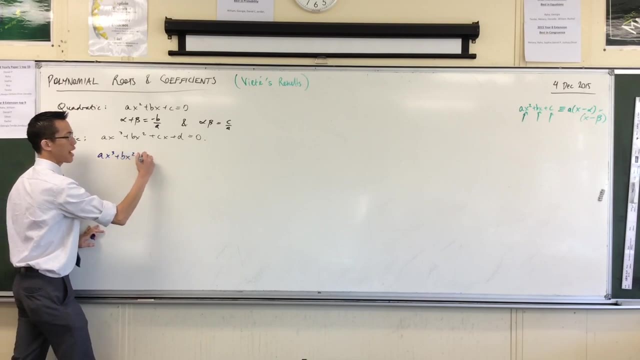 Three. It should have three, just like a quadratic has two. There should be three roots and I want to know how they relate to each of these coefficients. okay, So my method is going to be just like over there. I'm going to say: look, this thing here should be equivalent to something which has three roots. 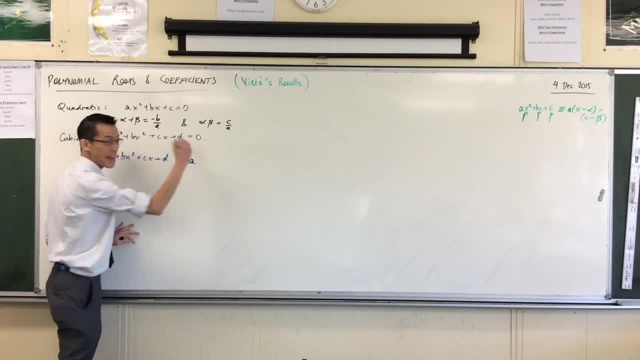 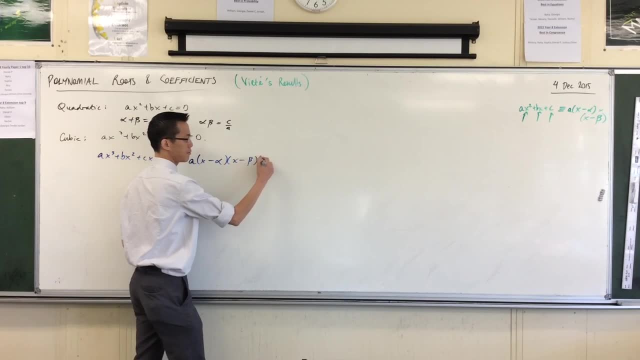 I want it completely factorized out. So I have that a out the front, because it's not necessarily monic. And then if there are three roots, I'm going to call them alpha, beta and gamma. okay, In case you're wondering gamma, I'll draw a nice big gamma over here. 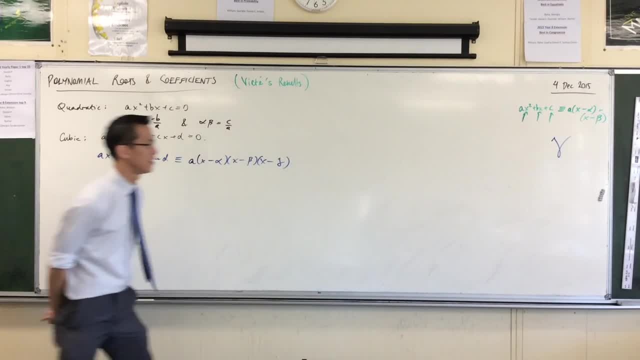 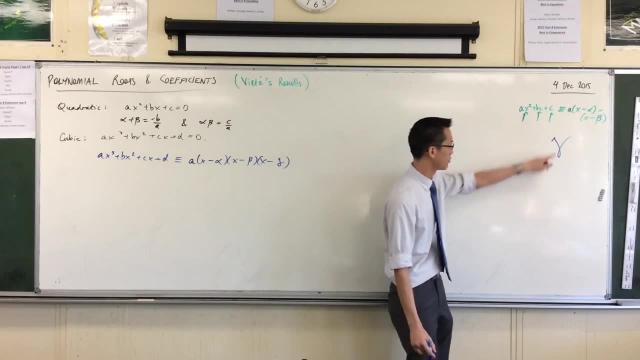 This is the way I draw gammas, okay. Kind of like a. how would you describe it? It's like a ribbon. You know those ribbons that you buy, the fundraising ribbons. It's like a ribbon with a tail, okay. 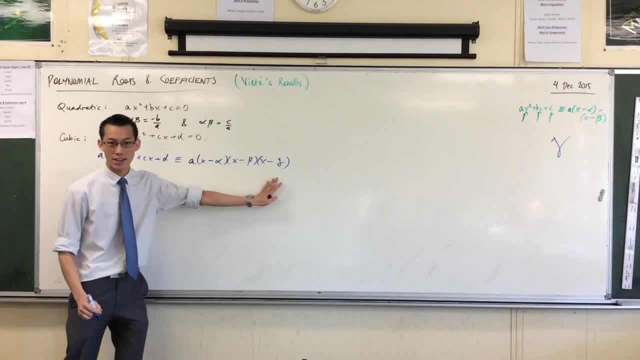 Or a hat, whatever it is okay. So here's my factorization. Now I'm going to take this. I'm just going to expand the lot. okay, Now I'm going to give you a second. Excuse me. 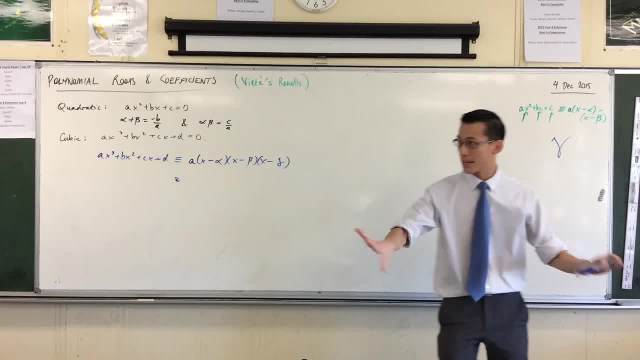 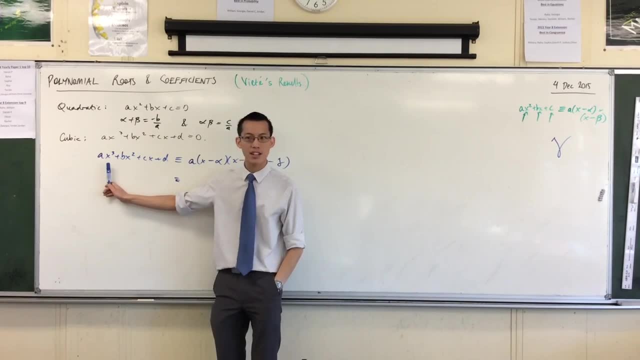 You're going to get a whole bunch of terms out of this. okay, Get all the terms out just one by one. It might take you a couple of lines, But the important thing that I want you to get is: can you gather the x cubed terms? 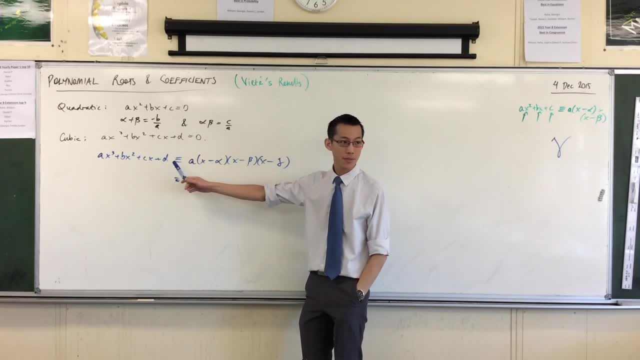 Can you gather the x squared terms? Can you gather the et cetera? okay, Now just to make things one step easier for you before you begin your expansion. okay, Before I expand. can you see? everything here on the right is going to have an a on it, right? 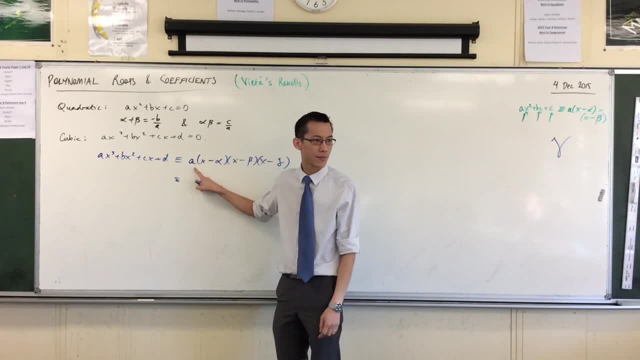 Like every single thing is going to have an a because there's an a out the front. okay, So rather than do that, I'm just going to take the a out of play. right, I'm going to divide both sides by a. 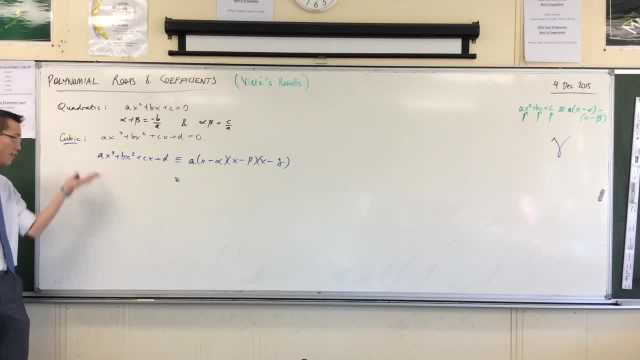 It's just a number. It's a non-zero number because it's a cubic. If a was zero, I'd have a quadratic. okay, So if I divide everything, I should get x cubed plus this number of x squared, plus this number of x's, plus this number of x's. 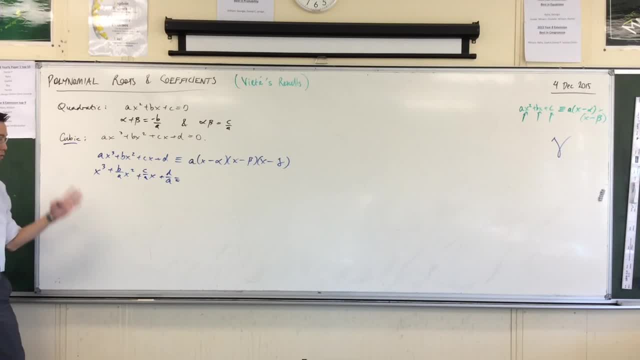 Okay, So I'm dividing that all by a, which just leaves me with this, which is no easier to expand, but there just won't be so many a's flying around, okay, So now you've got the right-hand side. 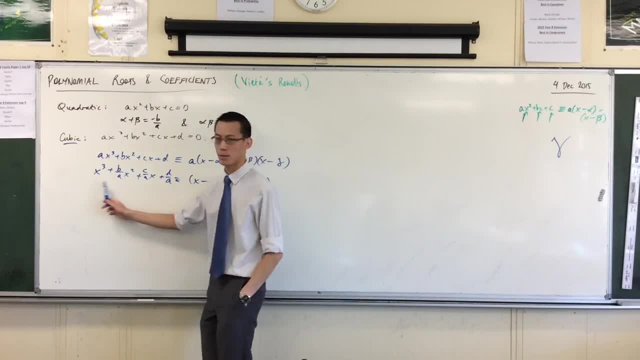 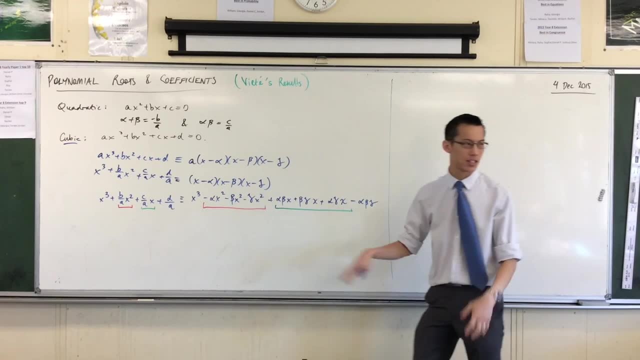 Go ahead and expand it and collect the like terms. okay, Off we go. I'm one step short. okay, You can see. what I've done is I've actually just expanded everything up, but I've put them into groups. I just haven't quite factorized yet, right? 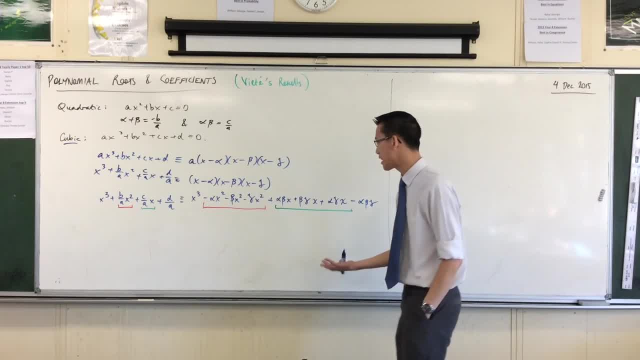 I'm pointing this out just so that you can see. Okay, Just to let you know. one of the tricky things here is just making sure you've got everything. Just make sure you haven't missed any terms. You're going to have three x squared terms. 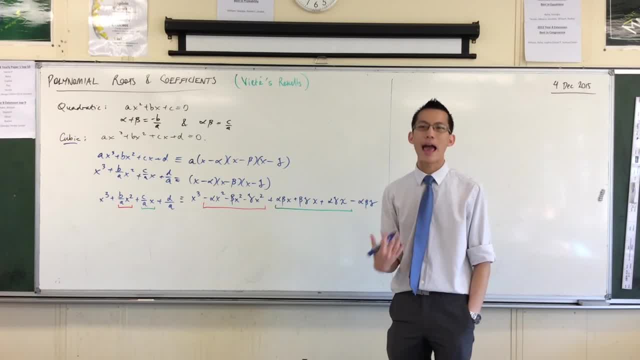 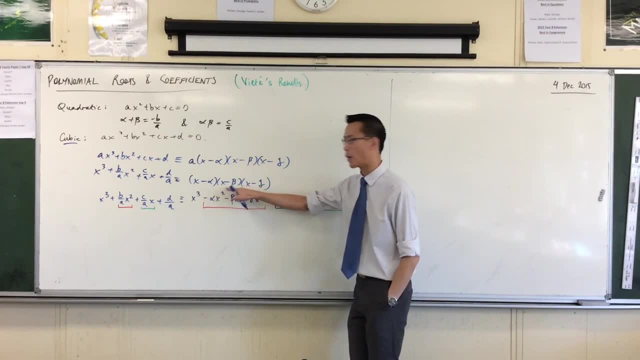 Now, just before I, you know, actually factorize this, how do I know I had to have three x squared terms? Like I knew I had to have three of them. okay, Have a look at how you get an x squared out of this, right. 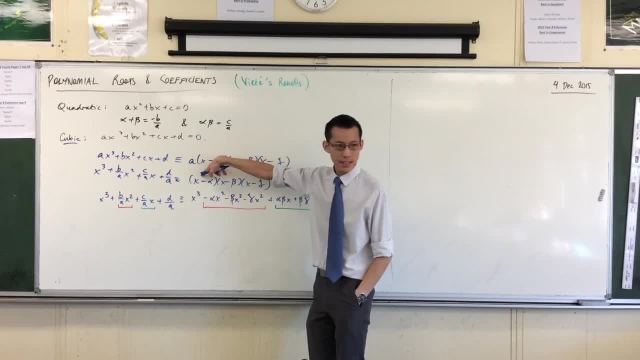 In what way could I get an x squared? And the answer is: you have to take these two, which leaves you with: well, don't pick an x here, because then you won't get an x squared, You'll get an x cubed, right. 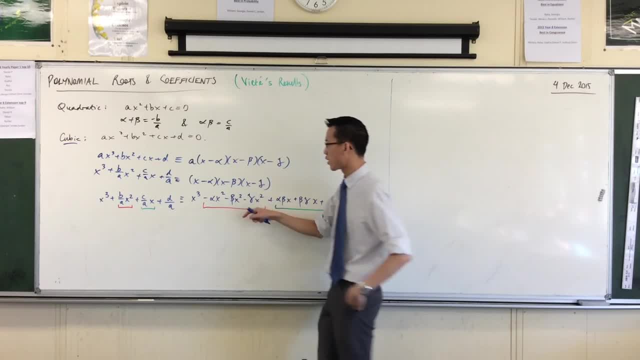 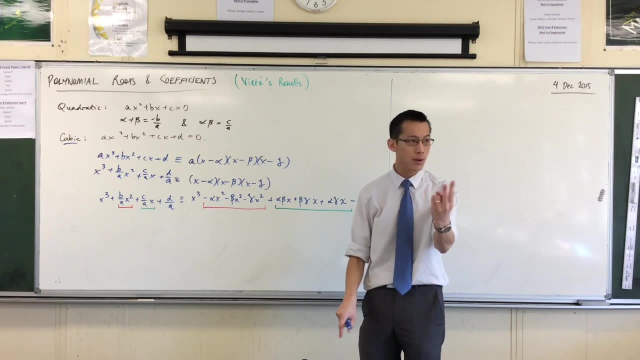 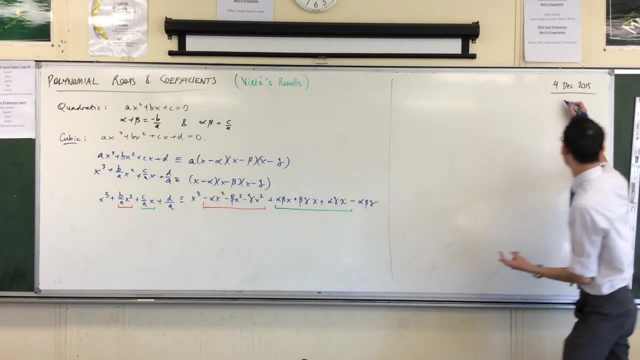 You've got to take these two, Then you've got to take these two, And then you've got to take those two right. In other words, out of three objects, you were trying to choose two of them right. In other words, thinking back to your binomial that you learned way at the start of the year, there were three. choose two of those right. 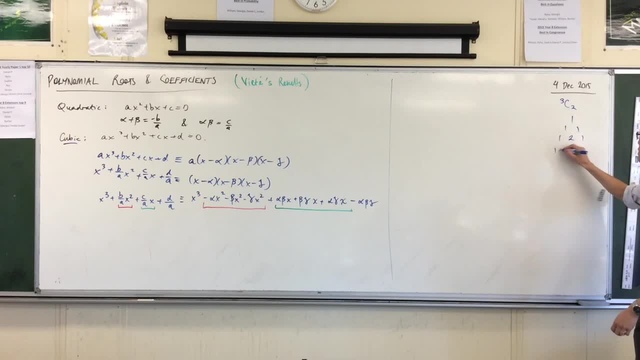 Which, if you want to go back to your Pascal's triangle right, Three choose two- is going to be able to do this. Three choose naught. Three choose one. Three choose two. Okay, So that's how I knew there were going to be three. 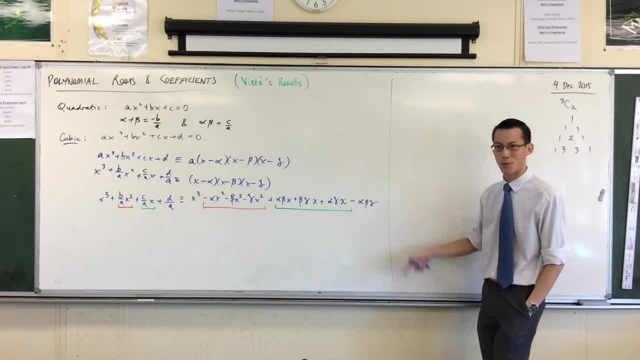 And your calculator can check that. Okay, That'll be more useful when we go to four in a minute. So I also knew there were going to be three of these. In fact, you can see the one: three, three, one that Pascal's triangle expected us to get. 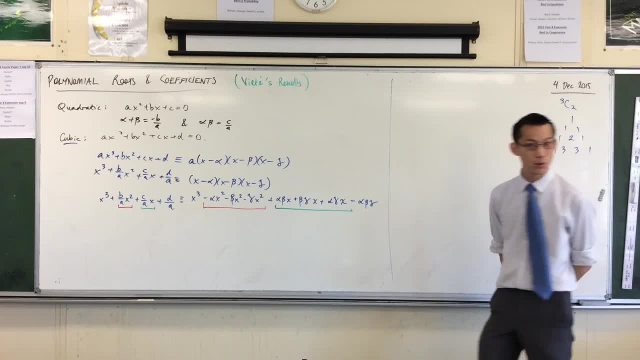 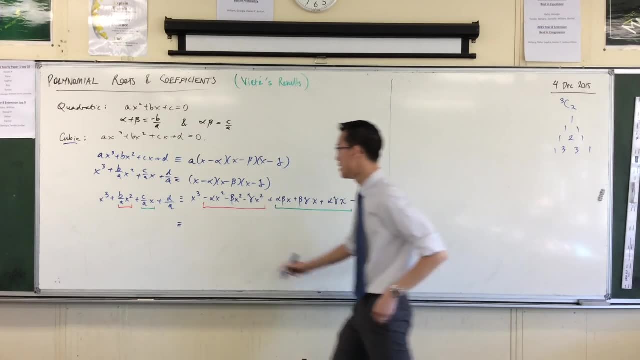 Okay, Do you see it? Okay? So, all right, Now I'm ready to factorize, So I'm going to. in order to make sure I can compare the coefficients, I need the actual coefficients. just sitting out the front, I notice there's an x cubed on both sides. 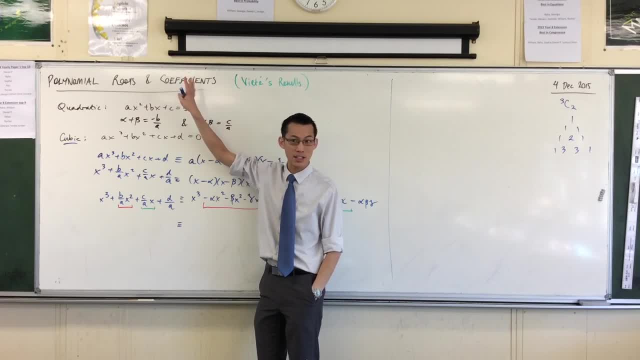 But that tells me nothing about the coefficients on the routine, How they're related to each other, So I'm just going to get rid of both of them. Do you see that It doesn't add any useful information to me? I've got an x cubed on both sides, but whatever. 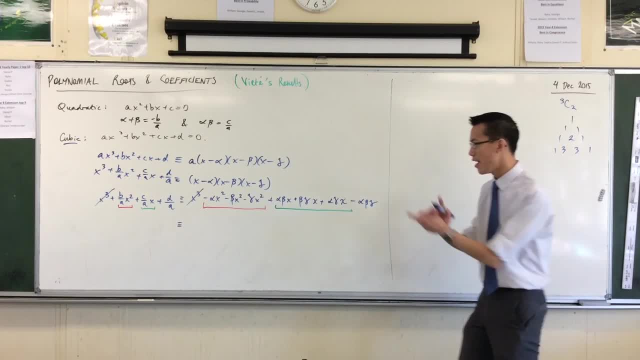 Okay, Now is here where the action happens. right, How many x squareds do I have? I'm going to take out that minus sign, because they all have a minus on them, And I get alpha plus beta plus gamma, Right, That's how many x squareds there are. 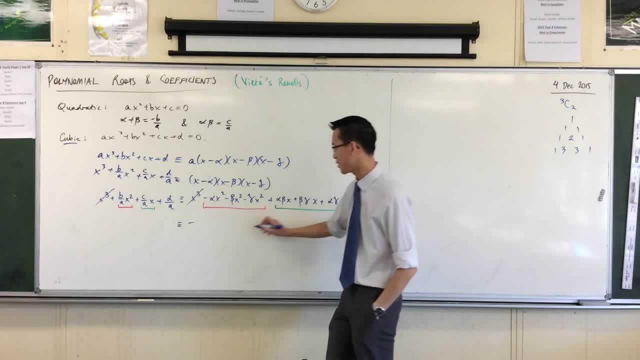 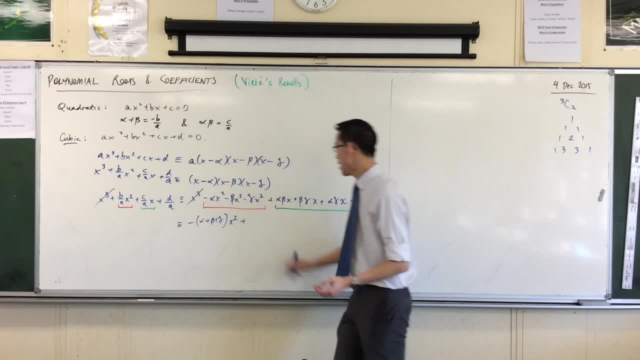 You can call them x squareds. There are the x squareds that are up In the same way. I've got all of these guys. Take out my factor of x. Bless you. Now these guys, what do you call them? 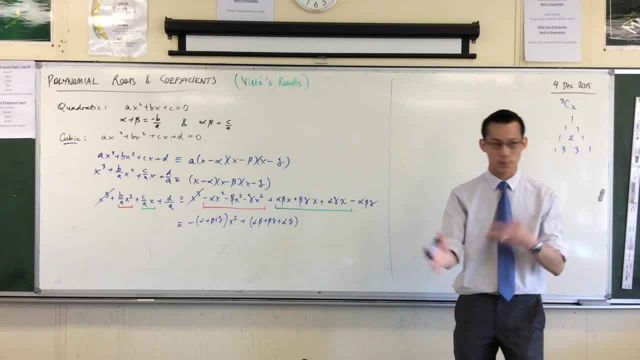 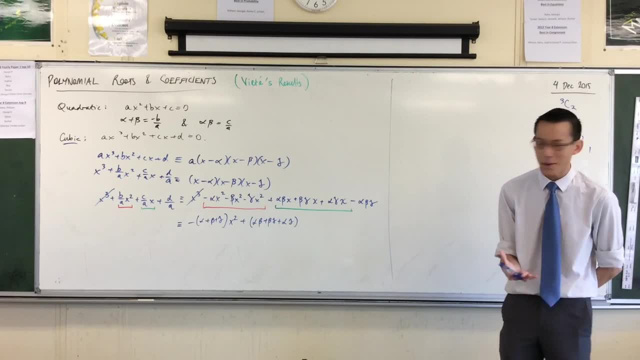 You cannot really call them the sum of roots, Because it's not alpha plus beta plus gamma, But you also can't call them the product of roots, because it's not alpha times. Okay, so what you call these is- And if I write the last one here, you can see there's a pattern that I can name these- 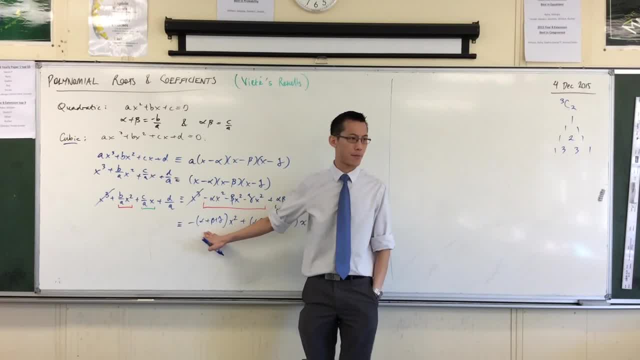 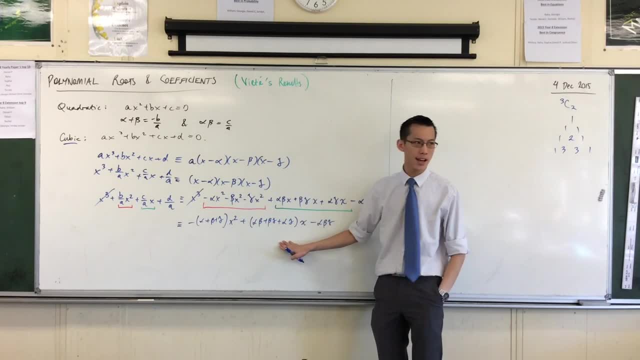 It will be consistent. sum of the roots, but it's the sum, one at a time, Just one root, then the other one, then the other one. This one is still a sum, It's something plus something equals something. But they're not one at a time, They're two at a time. You see them, They're all paired. 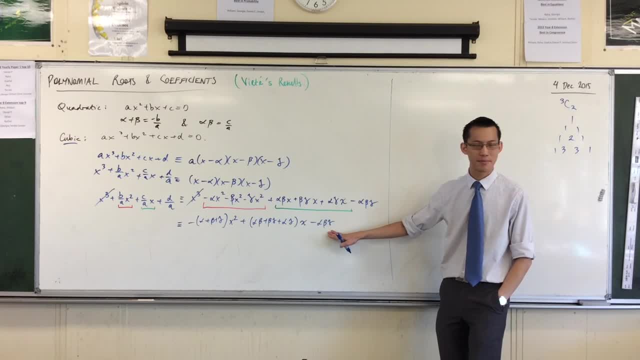 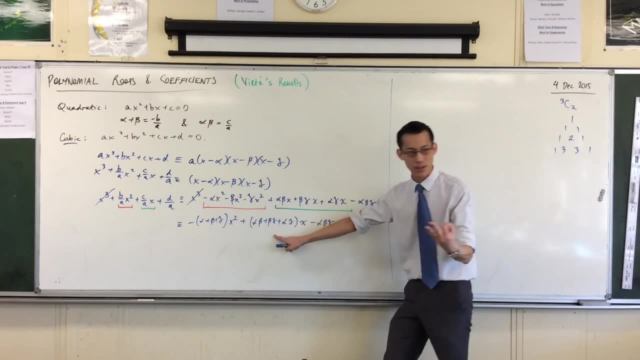 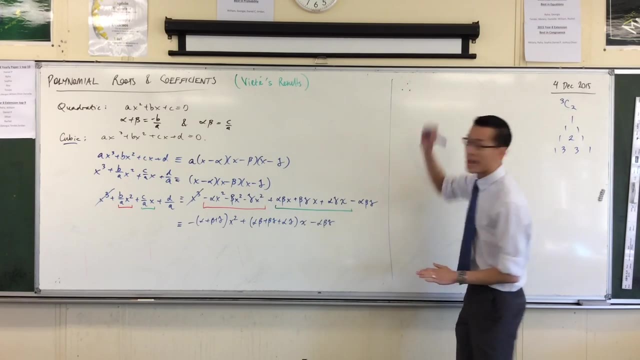 up. This is also a sum, but there just happens to be only one object there. It's the sum three at a time. So the sum one at a time, sum two at a time, sum three at a time, those are the coefficients that I'm actually getting and I can compare over there. So therefore, 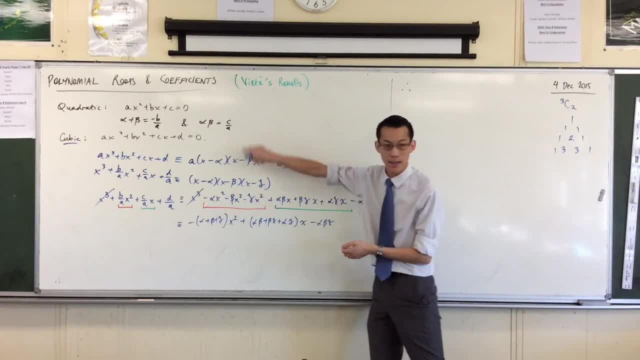 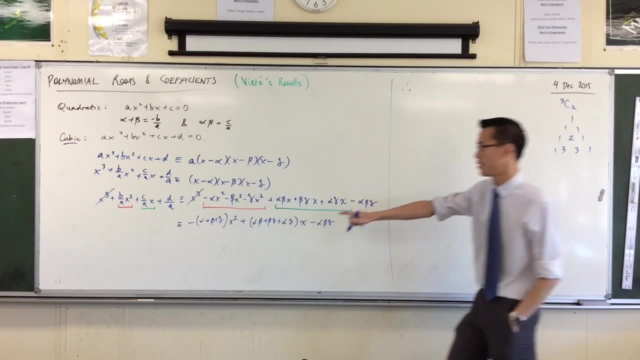 and here come the first of- or rather the second, because we've already got the first up here. Here come the second of Viette's results. He takes the coefficients and compares them. The first one is here. I've done the colors you can see again. but this makes 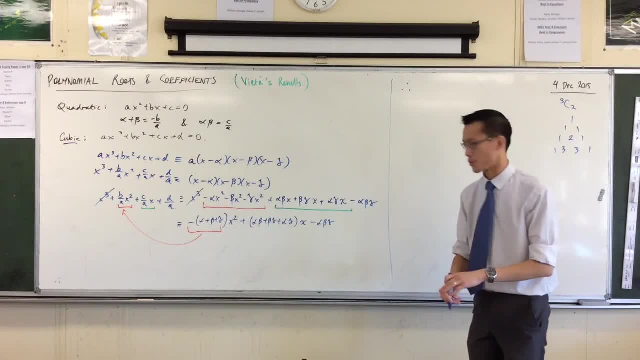 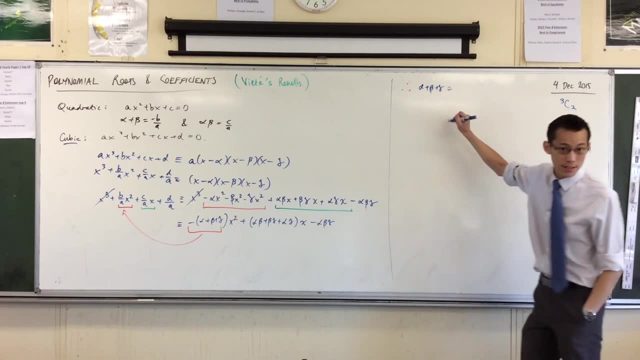 it a little more obvious. You've got minus alpha plus beta plus gamma equals b on a. So I'm going to put the minus sign on the other side, as is traditionally done. So there's the sum of roots and that minus sign pops on the other side, as you should. 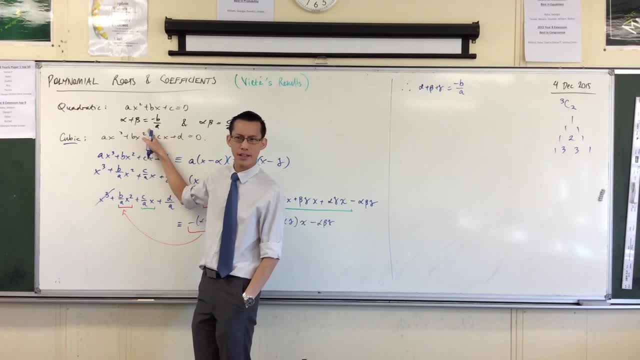 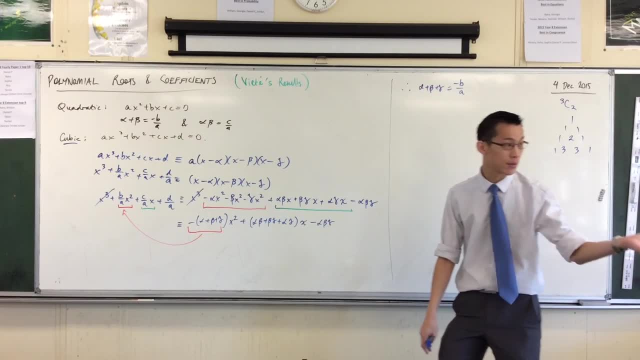 expect, based on this Interesting, No matter how many roots there are, no matter what degree your polynomial is, if you add up all of the roots, you'll always get this result. The next one is two at a time. so you go: alpha, beta, beta gamma, alpha gamma. That's just. 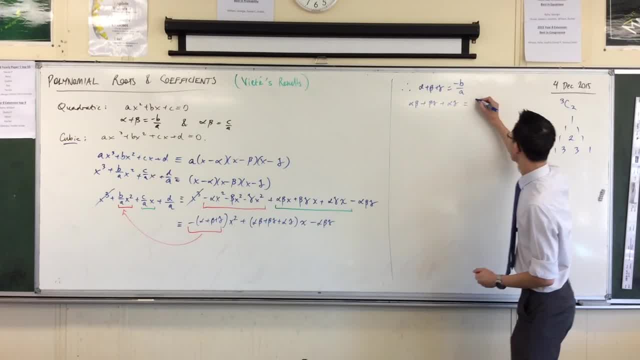 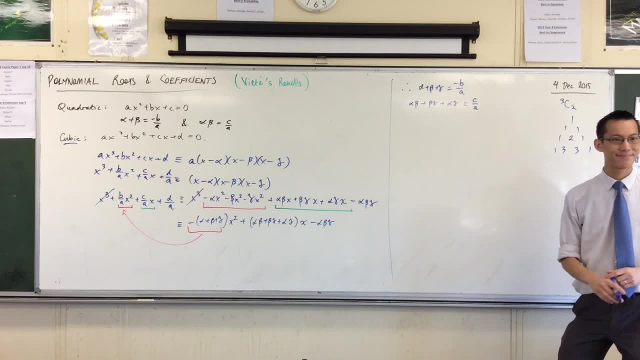 here and here there's no change of sign required. OK, so that's c on a, And then lastly, the sum three at a time. Yeah, Is it minus b on a all the time? because on Pascal's triangle, like it always has. 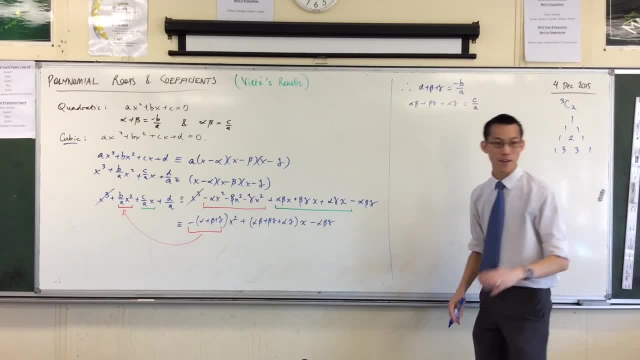 no number on it. You're not that far off. You're not that far off. When we look to four, you'll see what happens. OK, Let me write down this last one for the cubic. OK, so this is going to. 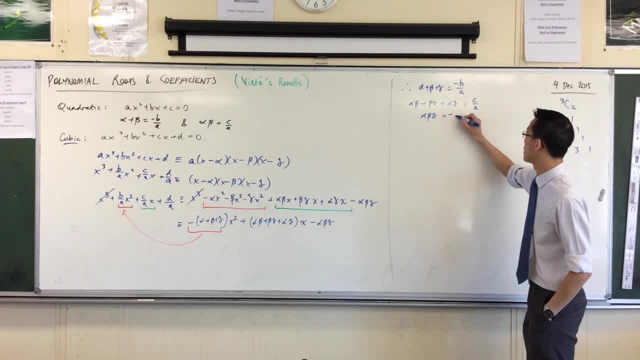 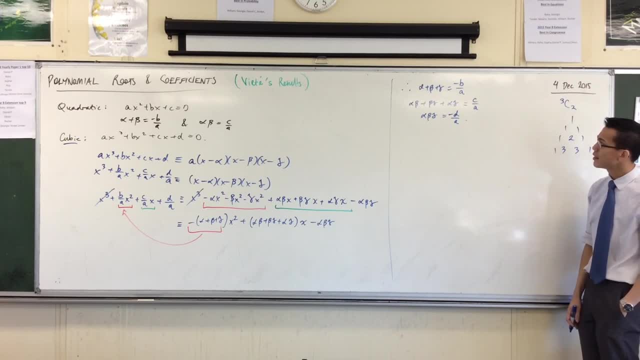 be again the sign It switches right. So you're getting minus d on a And these are Viette's results for the cubic equation. OK, So again you can see, just like we observed here, like it's actually the same numbers. 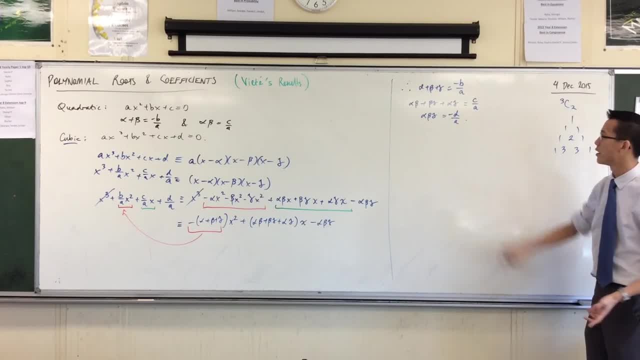 It's the same numbers and they're also alternating in sign. OK.